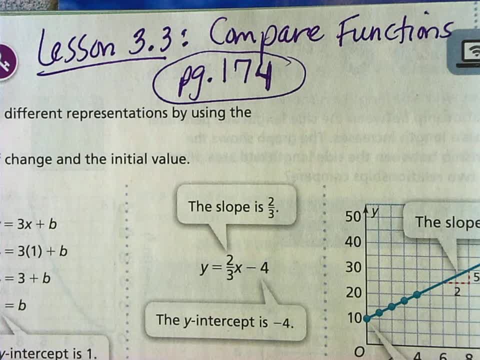 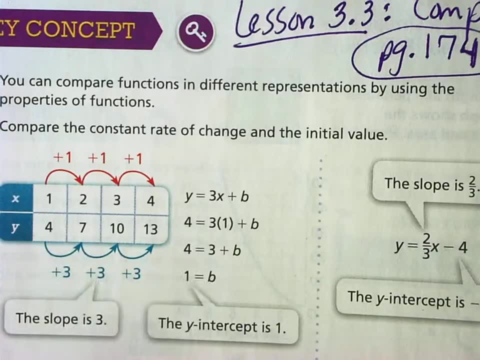 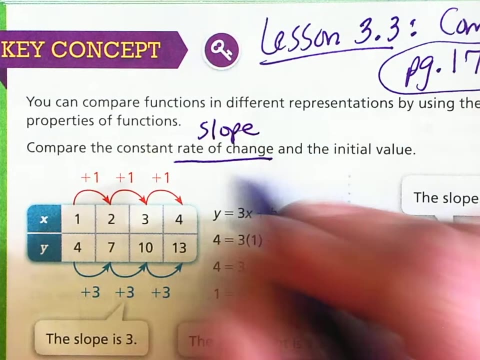 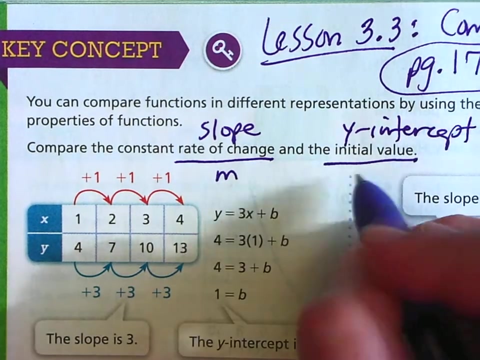 Hi there, Welcome back. Let's go over lesson 3.3, comparing linear and nonlinear functions. We're on page 174.. Okay so, remember, we are going to compare the rate of change, which is your slope, your m, and your initial value, which is your y-intercept, the b. Okay so here you can find. 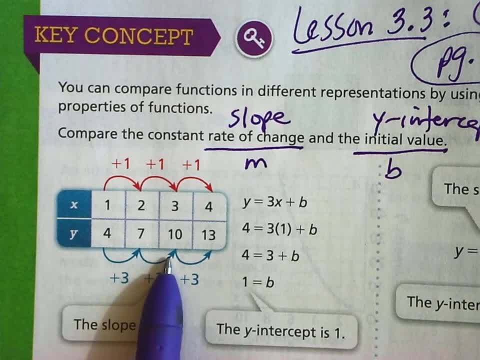 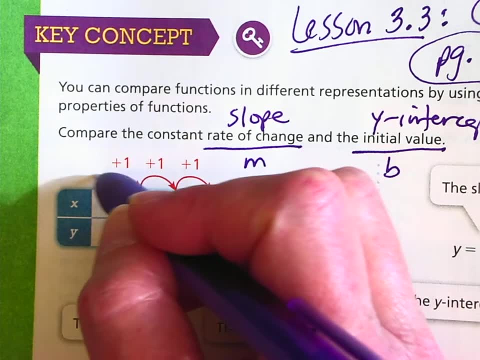 both. You can find slope and the y-intercept. Remember the y-intercept is when x is 0. So once you figure out your pattern in the numbers, you go back the pattern. So if you go back 1, you'll be at 0. And if you, the pattern here is going up by 3. So if you go back 3,. 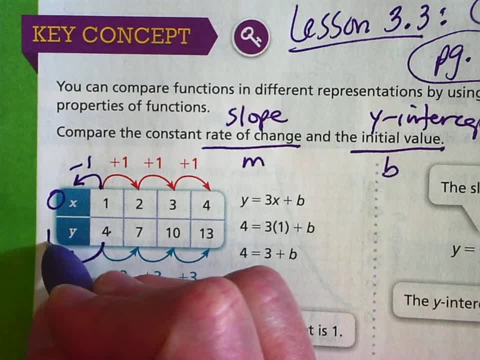 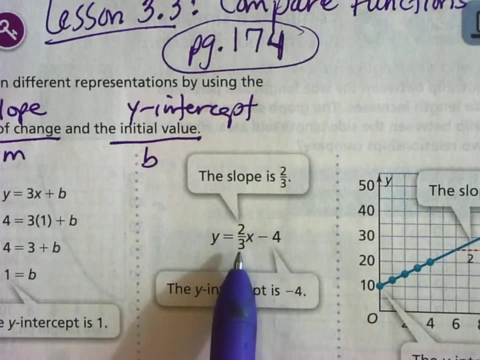 so back 3, 4, take away 3 would be 1.. There is your y-intercept: 1.. So we'll practice that. And then you have an equation. Remember: your rate of change is your slope and your. 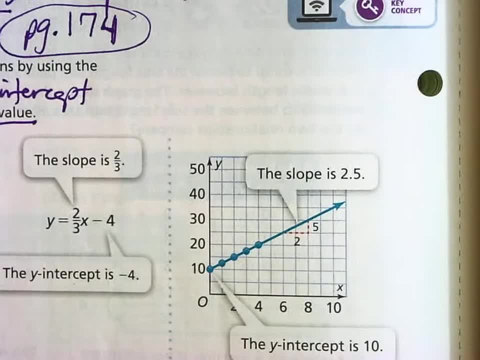 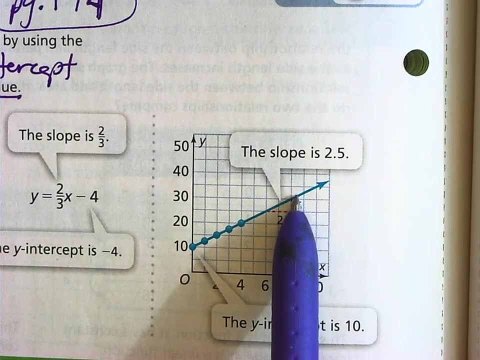 y-intercept is your initial value. And then again you can also find that here Again, your y-intercept is your initial value, where the line starts on the y-axis, And then your rate of change is how much you're going up or over, or down or over. So let's take a look at this first one. 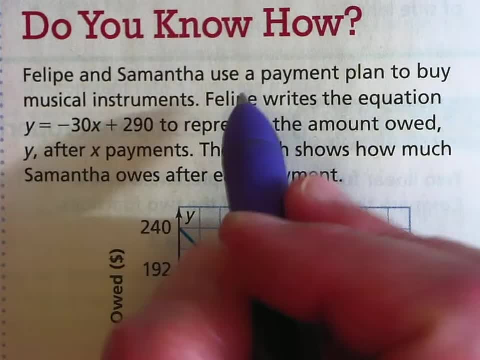 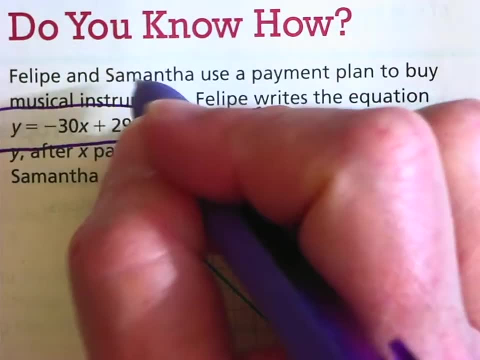 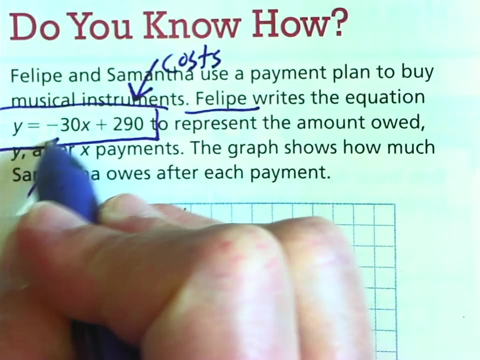 Felipe and Samantha use a payment plan to buy musical instruments. Felipe writes his equation like this: So that means he owes $290.. That's what his instrument costs. It costs $290, and he's paying $30 a month. That's what that part means. Okay, so Samantha is the graph. 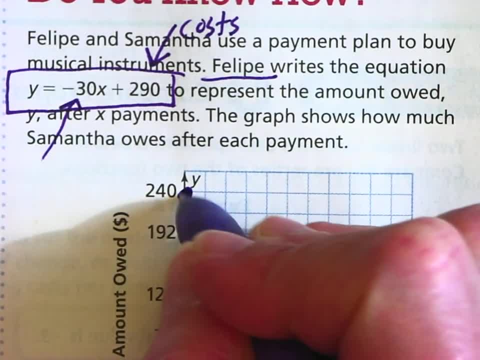 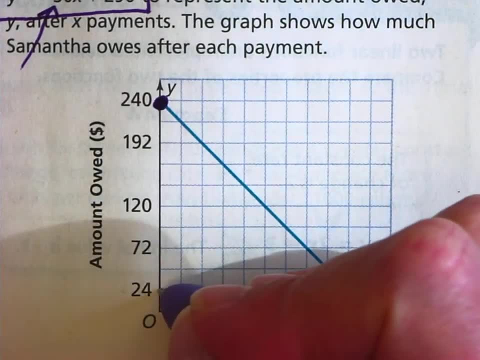 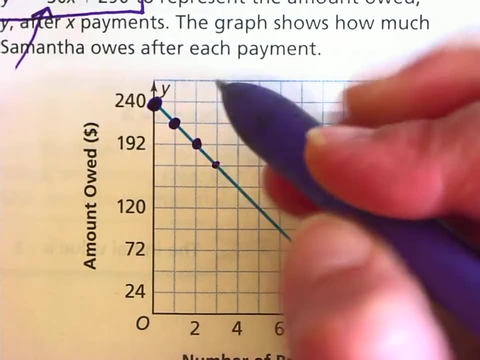 So her instrument costs $240.. That's where her amount starts. And then folks to figure out what she pays each month, look right here Every line is counting by 24, because it goes from 0 to 24.. So if you look at this, if every line is counting by 24, you're going down $24 and over. 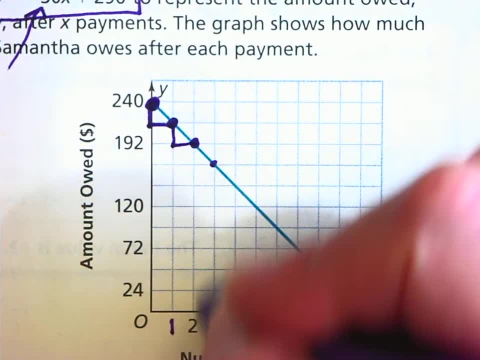 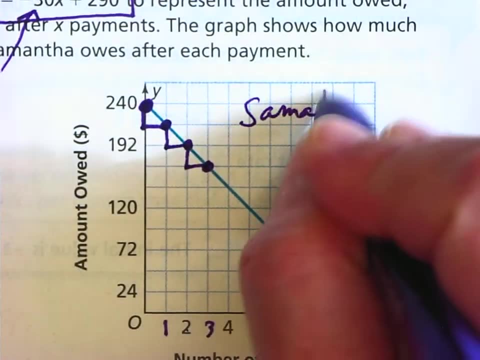 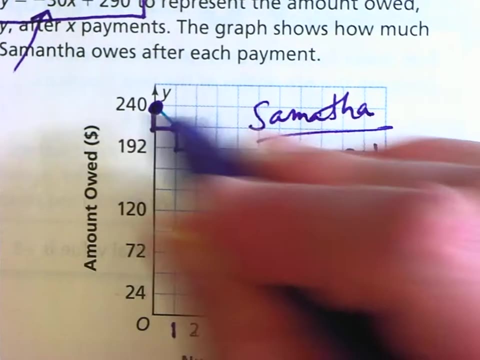 1. Down $24, over 1 each month. Down $24, over 1.. So the way you would write her, Samantha, her equation would be: y equals. so she's paying $24.. So she's paying $24 per month, plus her instrument started at $240.. So she paid $240. 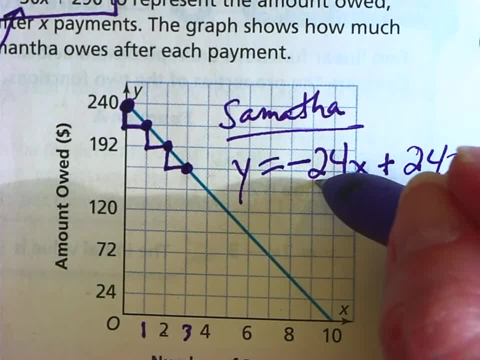 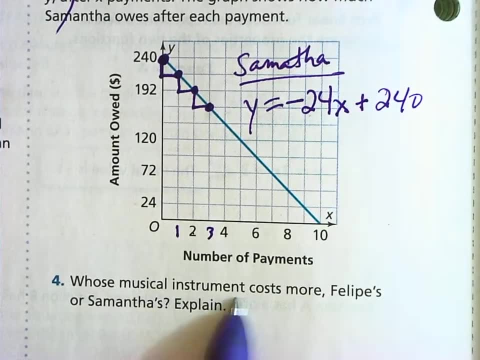 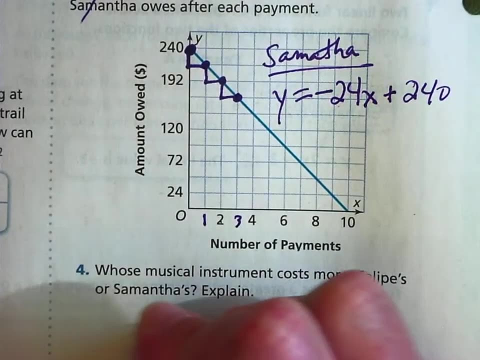 for the whole instrument, and hers is $24 a month, Whereas Felipe he paid $290 for his instrument and his is $30.. Okay, so whose instrument costs more, Felipe's or Samantha's? Well, Felipe's costs $290, and hers costs $240.. So Felipe's costs more. 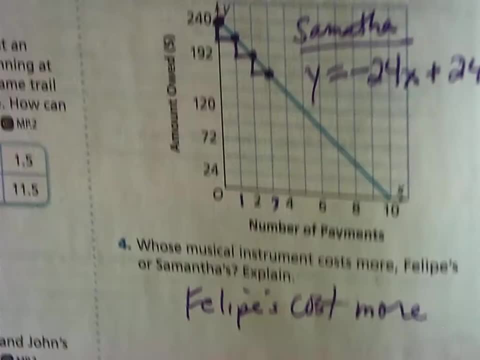 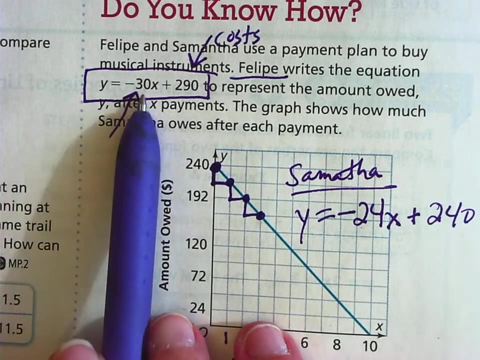 And then it says who will pay for the instrument. So she's paying $240 per month. who will pay more each month? That's part B. Who will pay more each month? Well, he pays $30 a month and she pays $24 a month. So he is paying more. 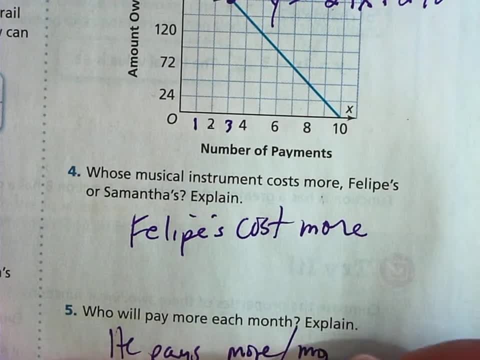 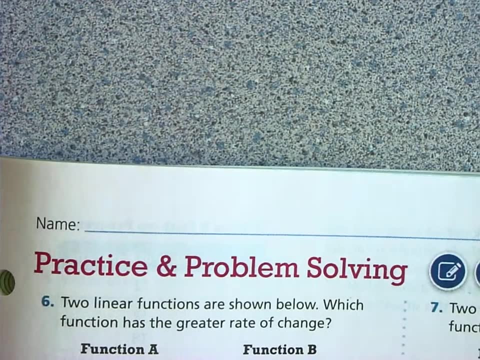 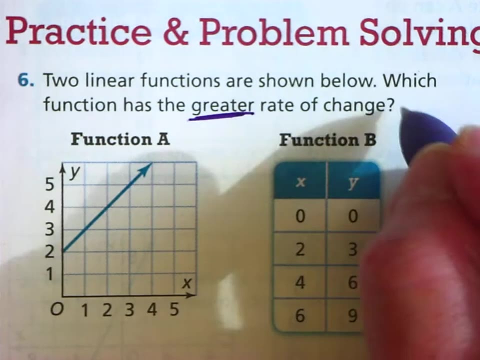 He pays more per month- $30 rather than $24.. Okay, so let's take a look at page 175 up at the top. Okay, so we're going to compare functions. now We're going to compare which function has the greater rate of change. Okay, rate of change is $240.. So we're going to compare functions now. 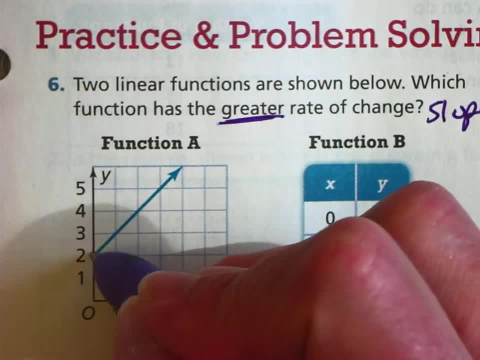 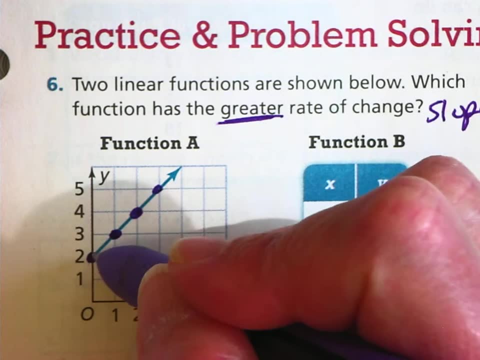 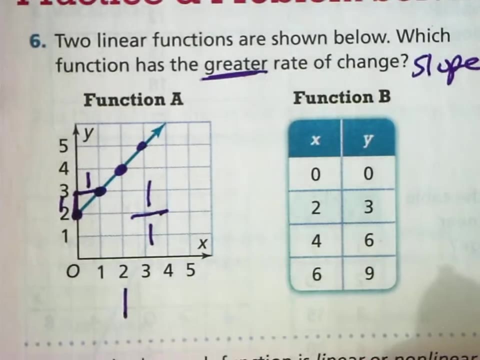 So if we start here and we rise and run, we figure out how much we're going up and over. So this is counting by ones, and this is counting by ones. So if we go up one over one, one over one is our slope, So this has a slope of one. Okay, so now this one. we don't have a line. 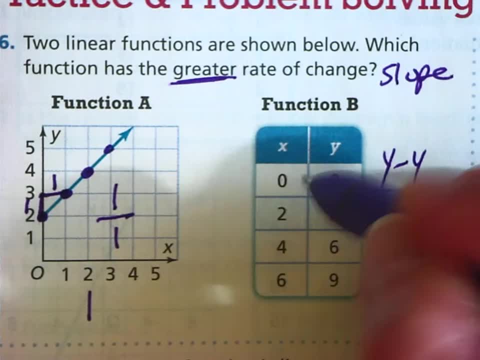 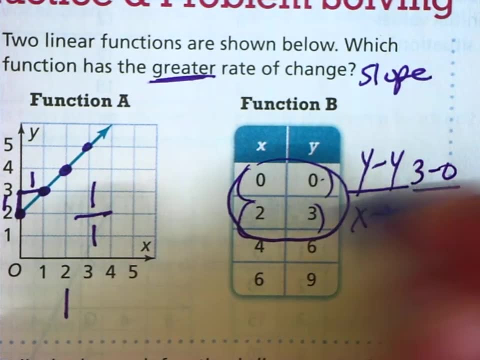 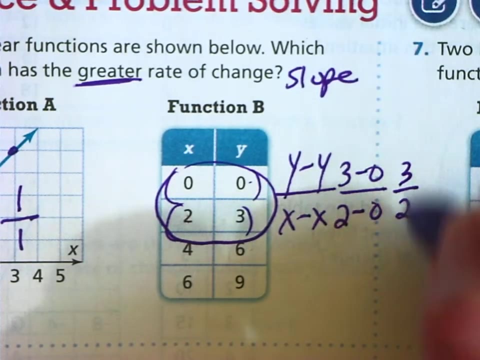 to look at. So we're going to use y minus y over x minus x. We're going to take two ordered pairs. Let's do this: one y minus y, so three minus zero Over x minus x. two minus zero, So three minus zero is three. Two minus zero is two Three over. 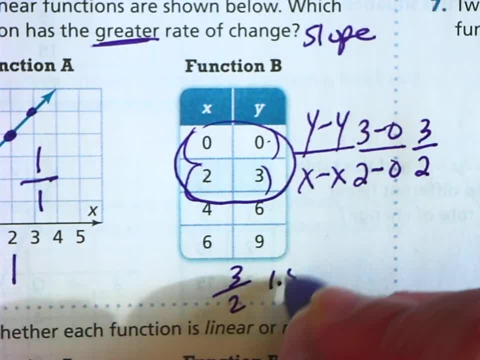 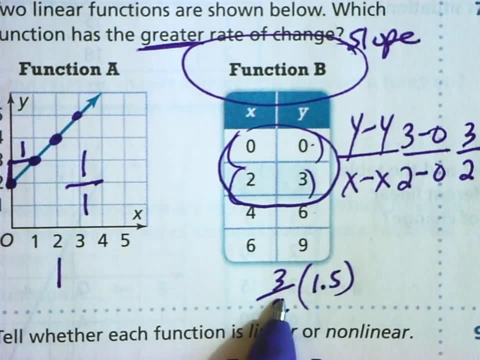 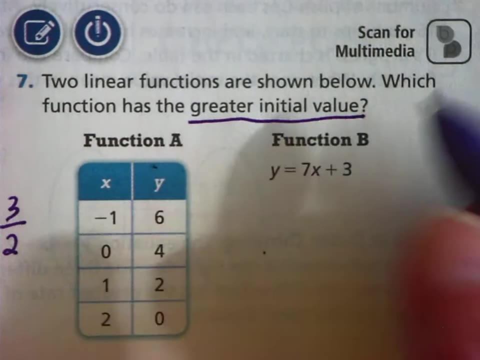 two is equivalent to one and a half. So which one has the greater rate of change? Function b, because it's three over two rather than one. Okay, so let's take a look at this next one, right next to number seven. Which one has the greater initial value? Okay, folks, that's the y-intercept. 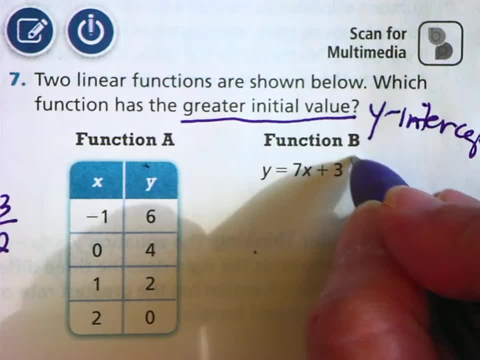 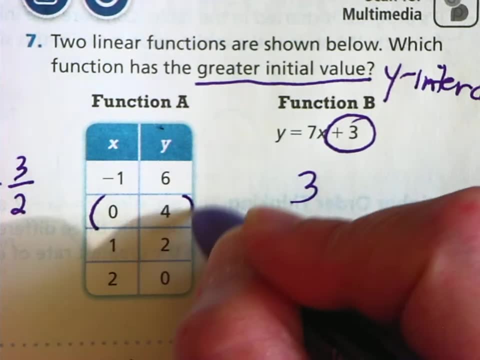 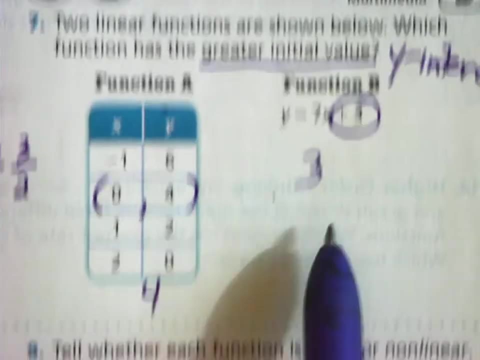 okay, so let's look at function b. the y-intercept would be three, and then the y-intercept for function a, folks, is the point that starts off with zero, something that is the point that's going to cross your y-axis. so the y-intercept for function a is four. so which one has the greater? 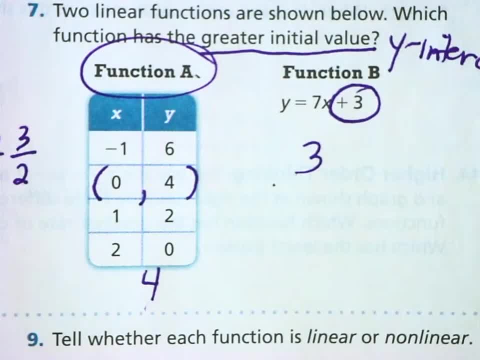 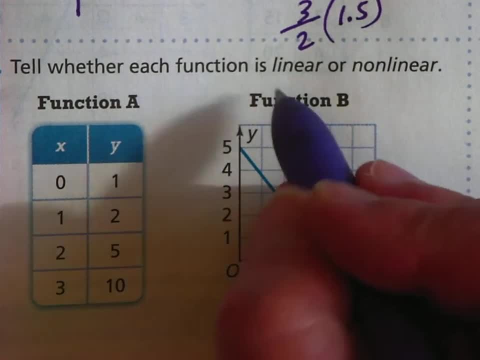 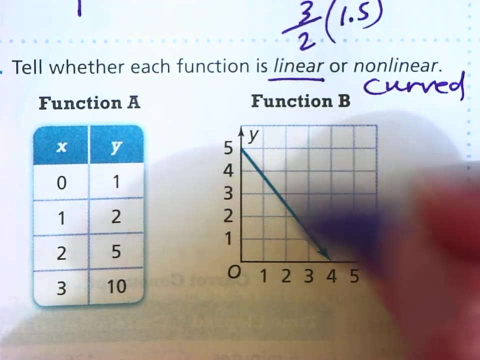 y-intercept: function a, because it's four, and function b is only three. okay, so let's take a look at number eight. tell which one is linear or non-linear folks. linear is a straight line, non-linear is curved. so function b folks, right off the bat, this is linear, it's a straight line. 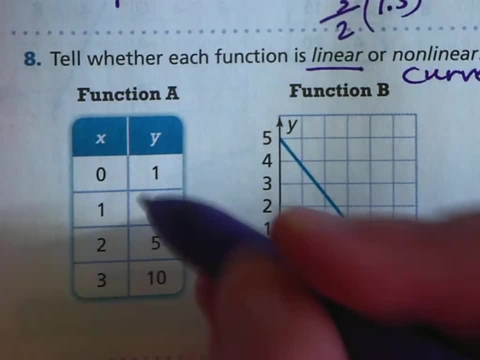 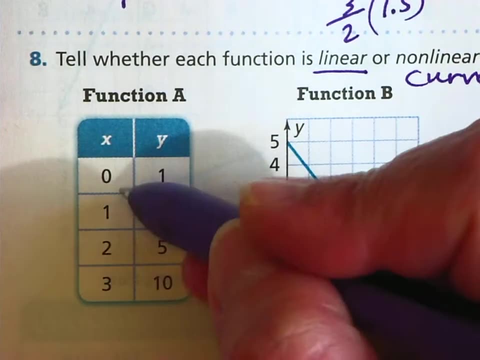 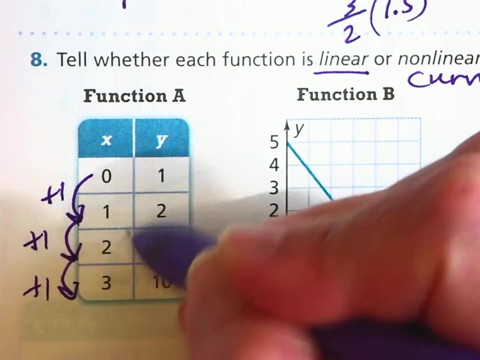 so that's linear. now the way to tell um if a function is linear or non-linear is it's going to be a straight line if it has a constant rate of change. so let's see if there's a pattern in these numbers: from zero to one is adding one, and then one to two, adding one. two to three, adding one. 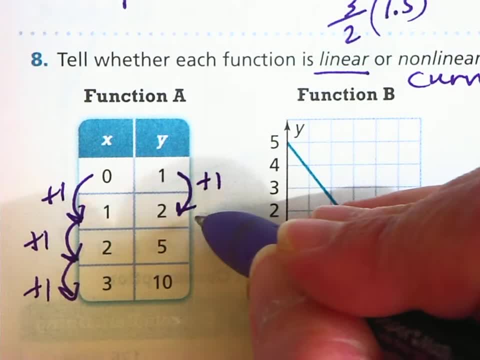 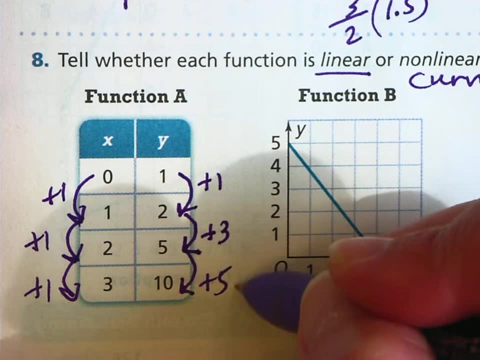 so that's a constant rate. but watch, from one to two is adding one, but then from two to five is adding three, and then from five to ten is adding five. that is not a constant rate of change, that is not a pattern. so this is going to be non-linear. there is no constant rate of change, it's not. 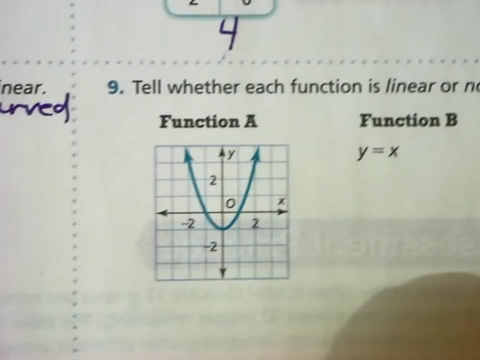 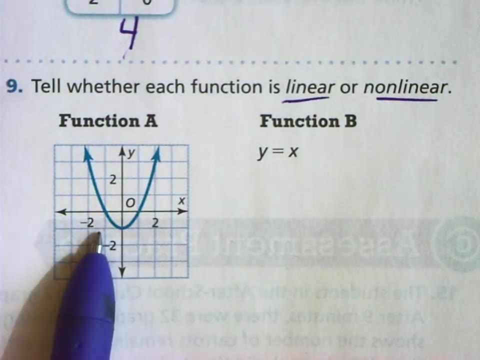 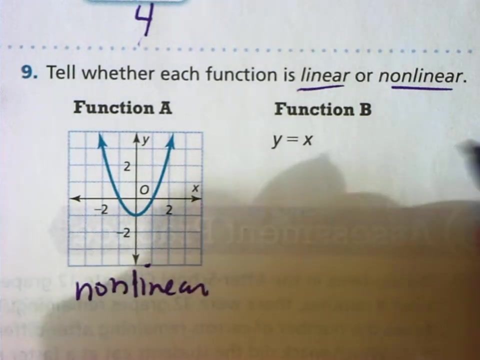 changing at the same rate. going to be a curved line, okay. so let's take a look at this next one. tell whether each function is linear or non-linear. again, okay so, folks, non-linear. look you, it's curved, it's a curved graph. so this is not straight non-linear. now any equation that is written in slope intercept form is going to be: 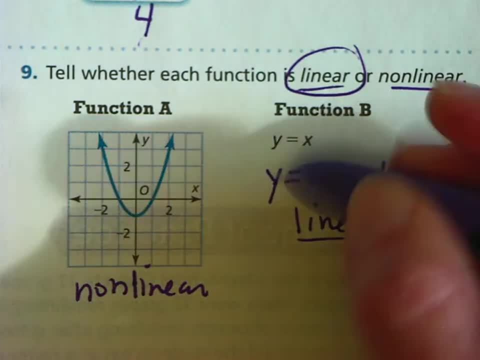 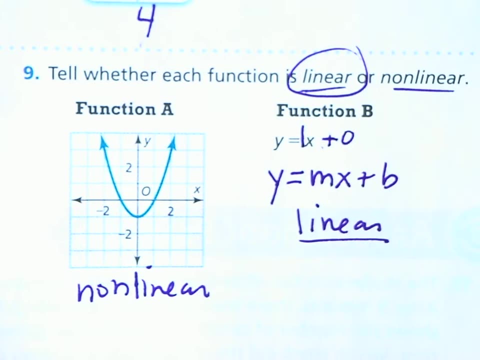 linear. so this one is going to be a straight line because the slope is one. and then look, the y intercept should be there and it's zero. there's nothing there. so that is slope intercept form. okay, so let's look at the next one: determine whether each function is linear or non-linear. 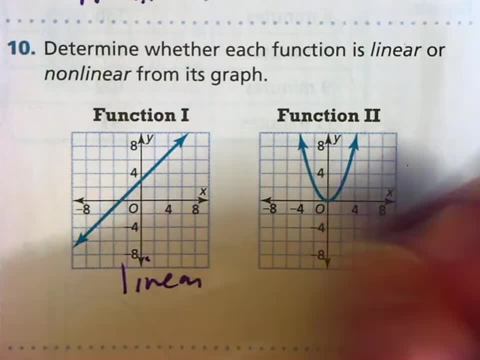 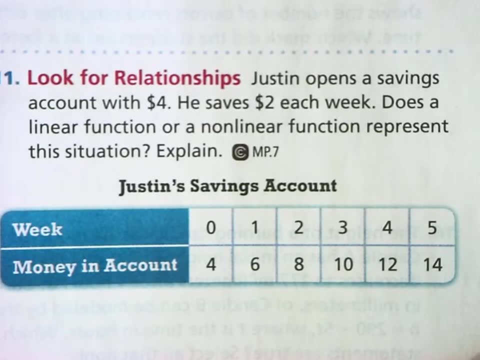 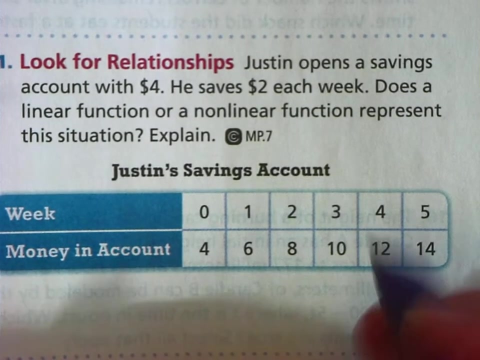 okay, folks, this is easy. straight line means linear. curved graph means not linear, non-linear. okay, let's look at this one. justin opens a saving account with four dollars. he saves two dollars a week. does it represent a linear or non-linear function? okay, folks, if it has a constant rate. 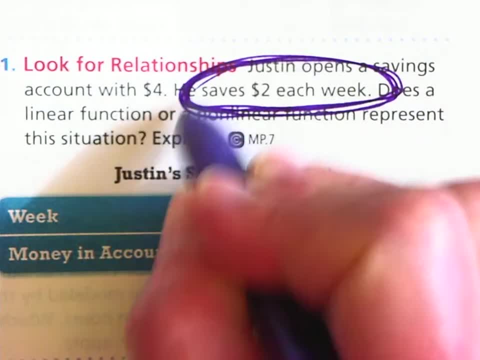 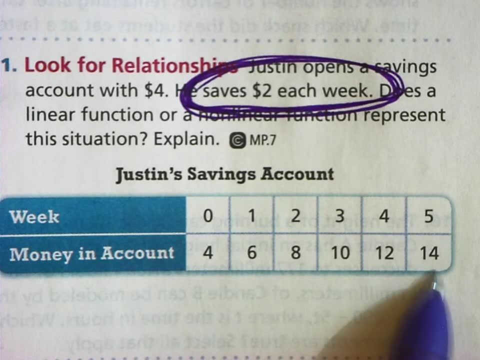 of change if the same thing is happening over and, over and over again. with the rate, it is going to be a straight line. so isn't he saving two dollars every week? every week, this is going up by two dollars. so this is going to be linear, okay, so now? um, let's take a look at this one. it's going to be. 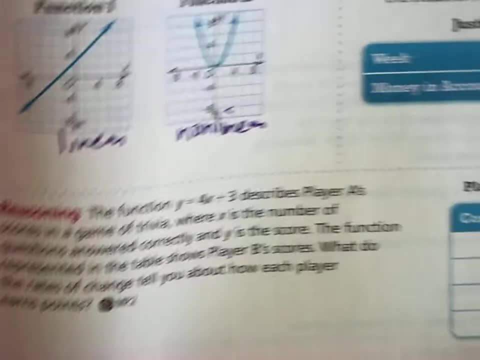 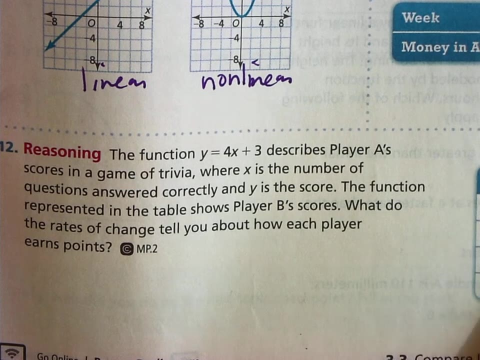 linear. so let's take a look at this one. the function for y equals four x plus c, describes players a scores and i gave him trivia. and then it says the function is represented for player b in the table. what do the rates of change tell you? okay, rate of change, the slope. so this player is. 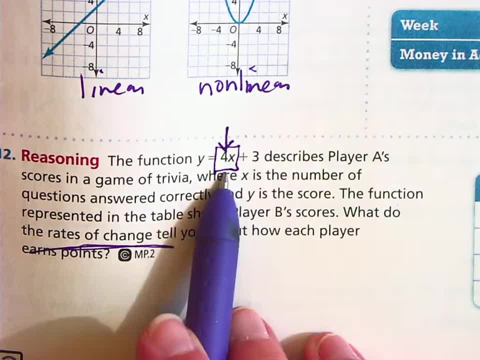 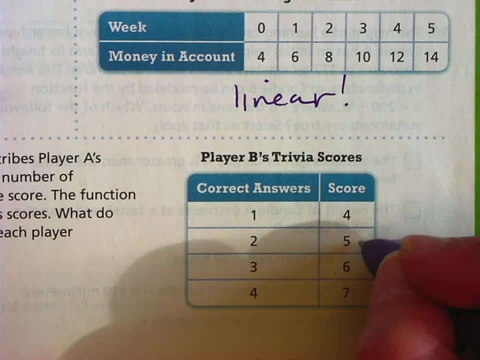 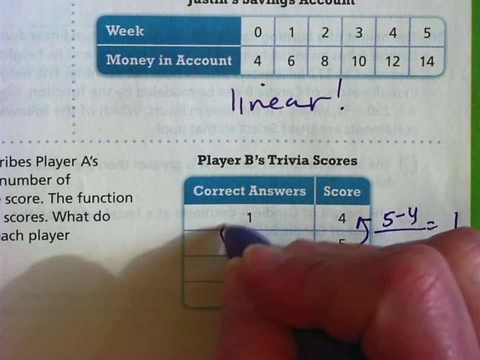 earning four points a question. that's the slope. four points a question. player b now rate of change. so y minus y, y minus y, so five minus four is one, and then x minus x, two minus one is one. so this one's earning one point per question. 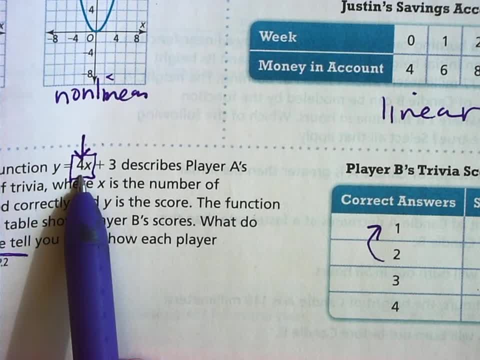 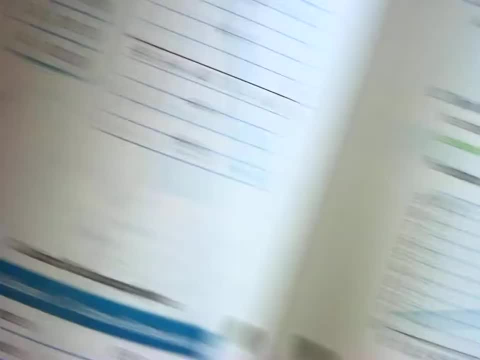 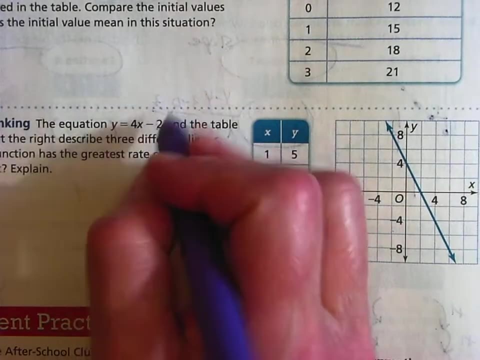 so player b- no sorry, player a earns more points per question- three more per question- than player b. that's what the rate of change tells us for this one. okay, folks, let's try to fit in one more problem. so number 14 on the back: okay, so you're actually comparing three different um things. an. 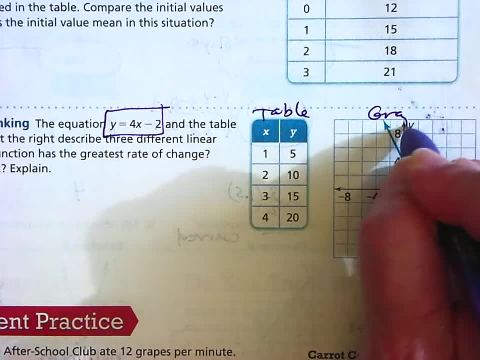 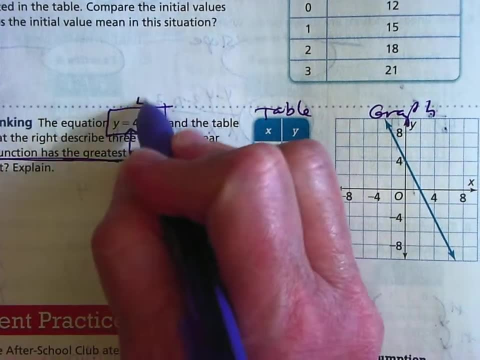 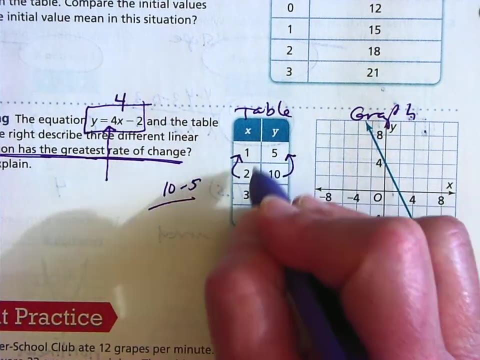 equation, a table and a graph. okay, so which function has the greatest rate of change? folks, the slope of this one is four. okay, let's do y minus y over x minus x, so 10 minus 5 over 2 minus 1, 10 minus 5. 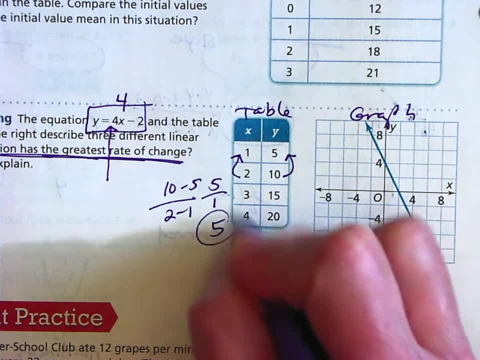 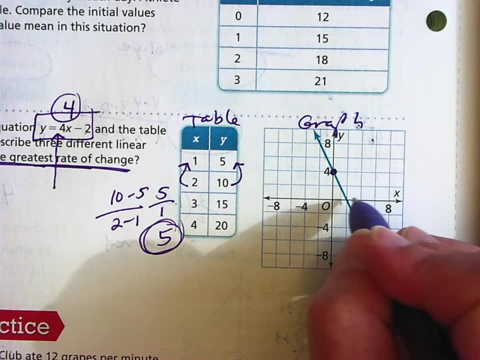 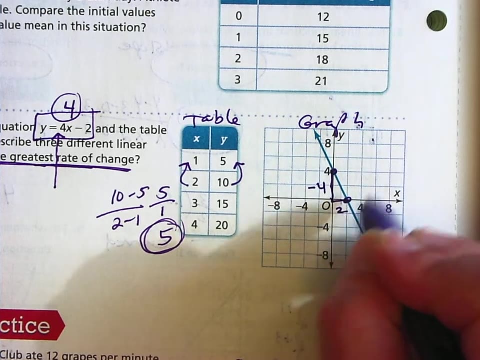 is 5. 2 minus 1 is 1. so 5 over 1 is 5. so this one has a slope of 4. this has a rate of change slope of 5, and then this slope is a negative slope. so look folks, i'm going every line's counting by 2. so i'm going down 2, 4 down, 4 over, 2 down, 4 over 2 is: 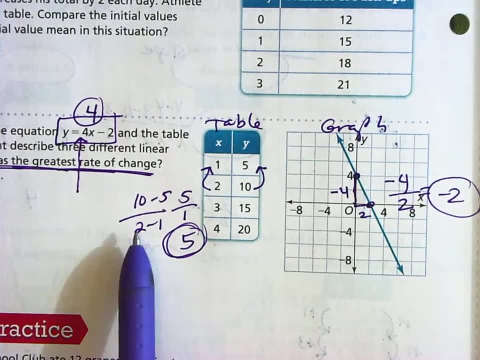 negative 2, so which one has the greater rate of change.